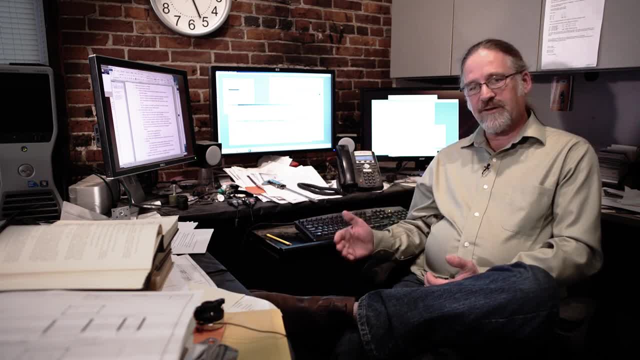 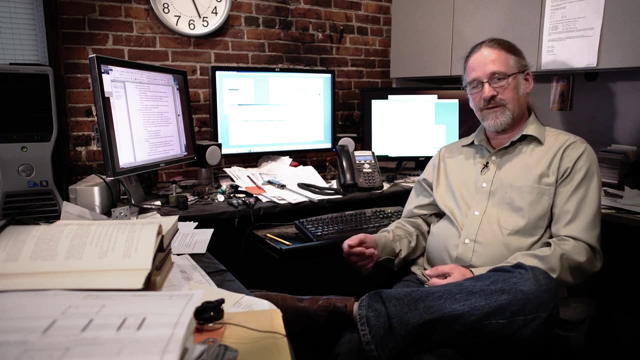 a purified impulse response. It's not an intuitive concept and it requires an understanding of FIR filters. I believe to understand how an FIR filter works, it's important to understand first how an IIR filter works and to see the difference. So I thought what I 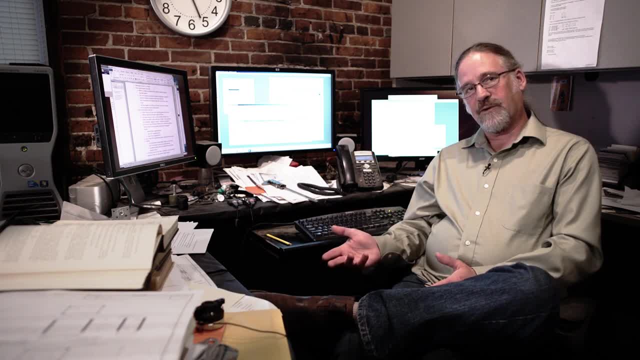 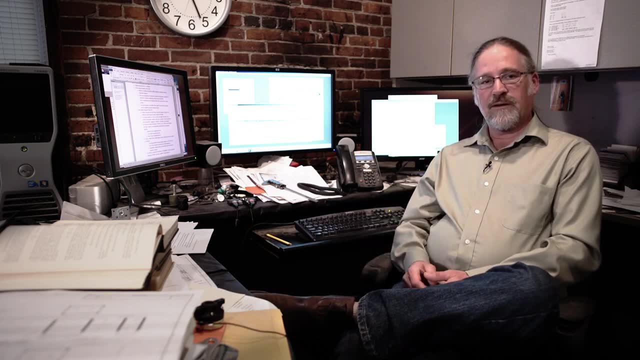 would do is explain how simple an IIR filter is, how simple an FIR filter is, and show the fundamental difference And then, with a simplified model of a smeared transient response, we can use a very simple FIR filter to purify that response. 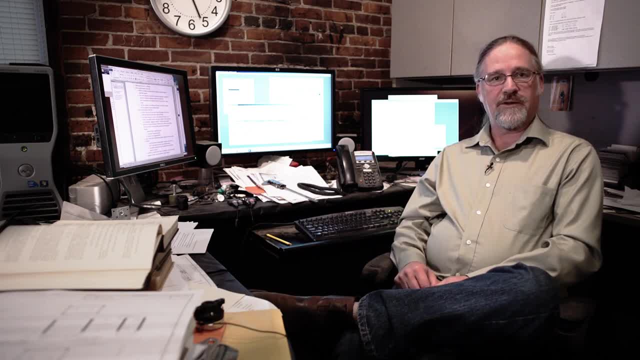 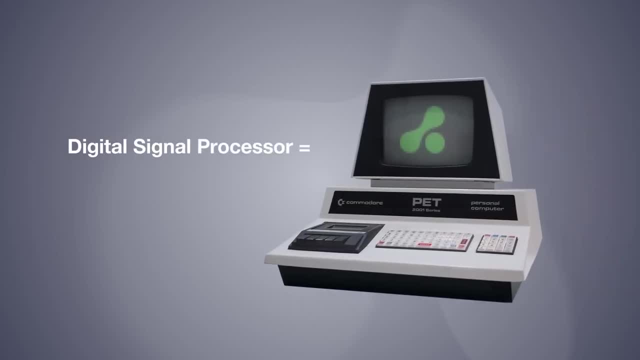 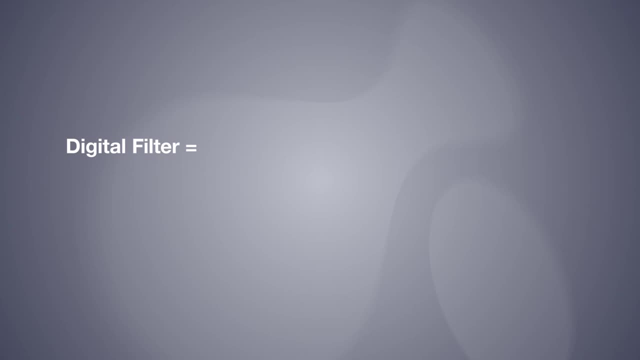 By extension That can be applied to a much more complicated loudspeaker impulse response. I'm sure everybody realizes that a digital signal processor is actually just a computer with specialized capabilities to do simple calculations very rapidly. A digital filter is a mathematical model of a physical system. To illustrate that I want to start out with 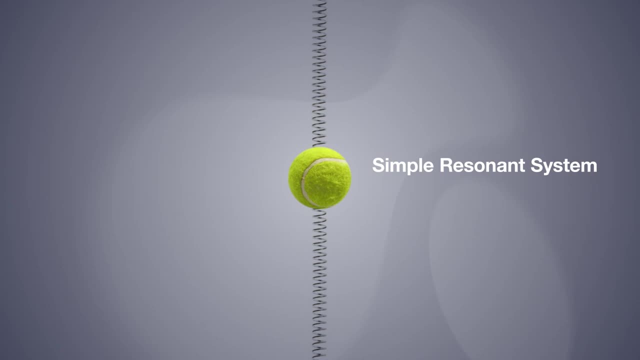 a very simple physical analogy, a simple resonant system which is just a digital signal processor. It's basically a ball supported on a spring. If we apply an impulsive input to this system by whacking the ball on the bottom, it responds by moving up and down in an oscillation with 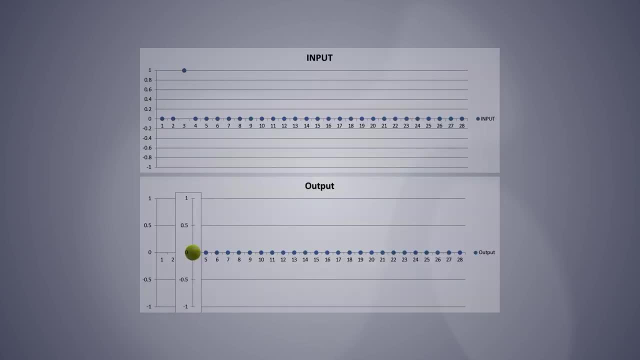 gradually decreasing amplitude. If we plot this motion against time, the graph we get is called the impulse response of the system. Whacking it on the bottom was an impulse and the response of the ball in terms of its position is the impulse response. Now, if we know the weight of the ball, the spring constant of the suspension and the 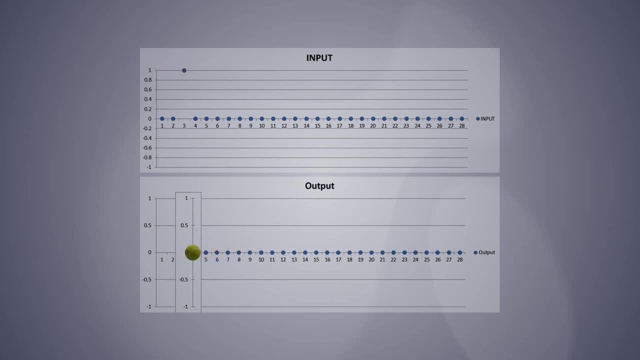 amount of friction. we have all the information we need to mathematically predict the position of the ball at any point in time after the impulse is applied. We don't have to calculate the entire response of the ball in one go. We can do the calculation sample by sample. 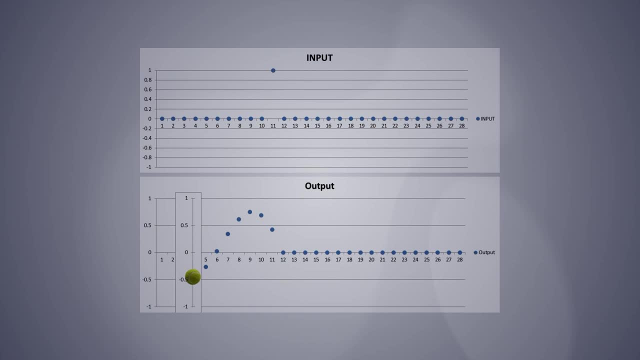 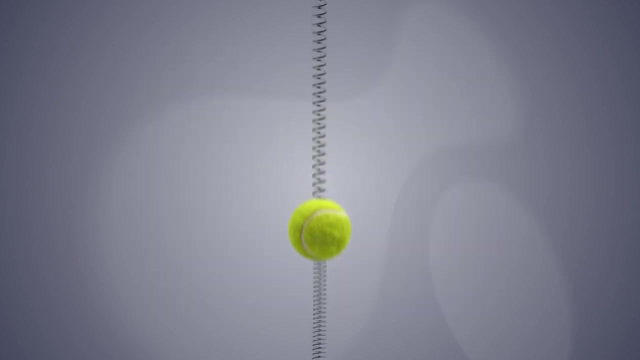 Let's freeze the animation here and look at the situation from the point of view of one sample. To calculate the position at the next sample, we need to know the current position of the ball and its velocity. The momentum of the ball tries to keep it going in the 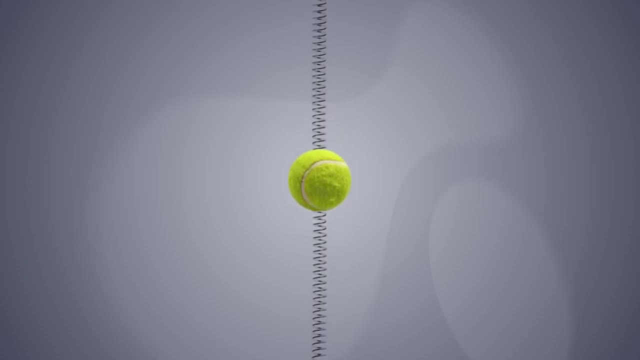 same direction at the same speed. The force of the spring accelerates it toward the center point or the equilibrium at the middle, and the resistance, the friction, always tries to slow the ball down. If we account for those three things, then we can calculate both the position and velocity. 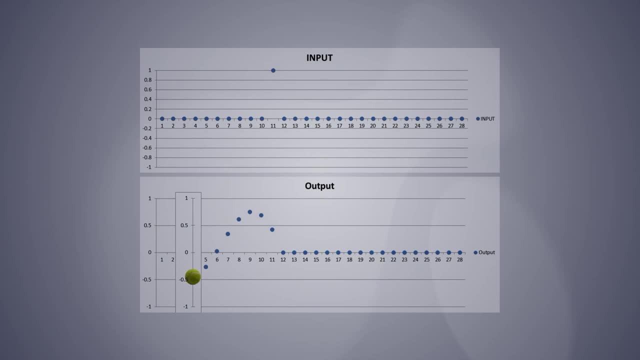 at the next point. So at this point we know the position. How do we determine the velocity? Well, we just need to look at where the ball was. the sample before The change in position, divided by the time, is the average velocity of the ball during that interval. 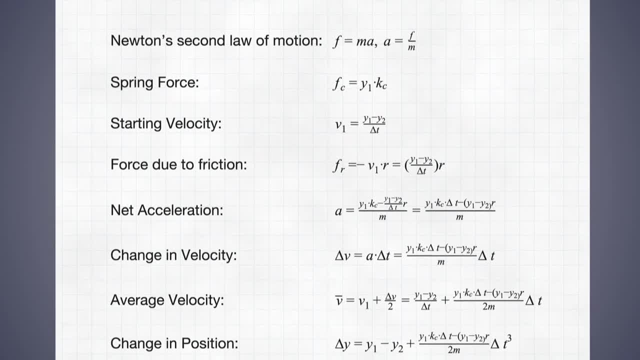 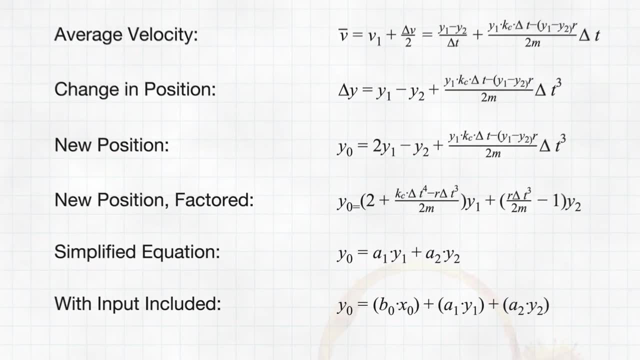 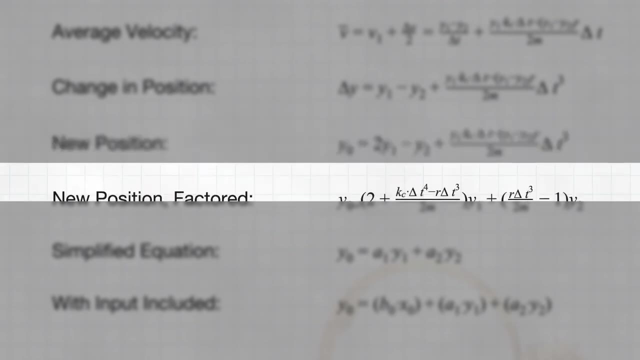 While the equations used to predict the motion of the ball are complicated, we don't have to go through all of them for each sample point. We can algebraically combine the equations into one equation, which is a complicated equation, reduce it to its most simple possible. 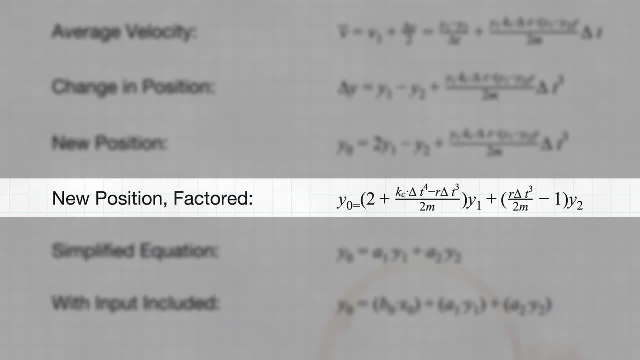 form and what we end up with is actually more simple than it looks. Everything inside the parents in this equation is a constant. You have m, which is the mass, you have r, you have k, which is the spring constant, and you have delta t, which, as long as our 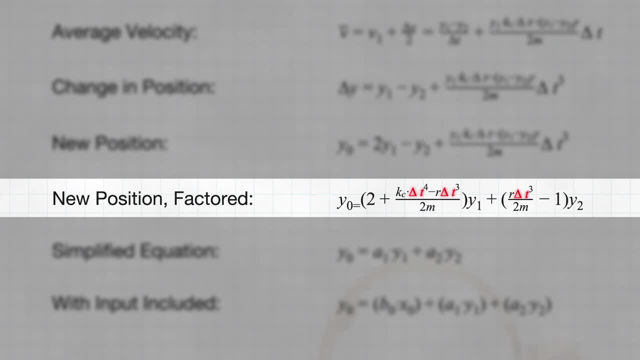 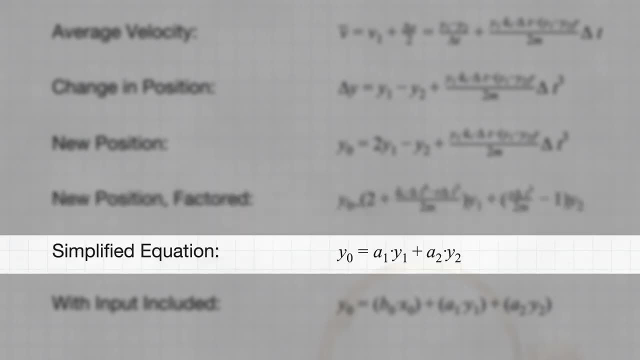 samples are evenly spaced is also a constant, So we don't have to do all the calculations inside the parents at each sample point. We can do that once before we start and then save the result inside the parents as a constant. We call it coefficient and the two coefficients 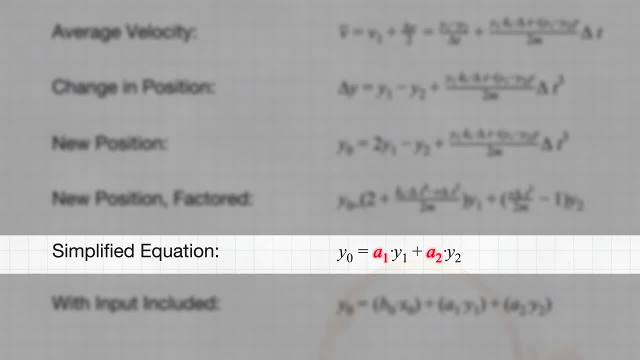 in this case will be labeled a, So we can do the math inside the parents and save the results. We end up with a very simple equation with two previous positions and two constants to capture everything we need to know about the weight, spring constant and friction To calculate the next position. 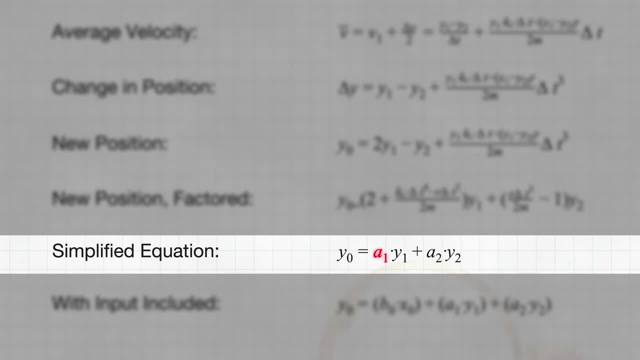 all we have to do is multiply the first coefficient, called a1, by the current position, multiply the second coefficient- a2, by the previous position, and then add the two results. There's our next position. So we've captured the resonant decay of this system, but we still don't have an input to. 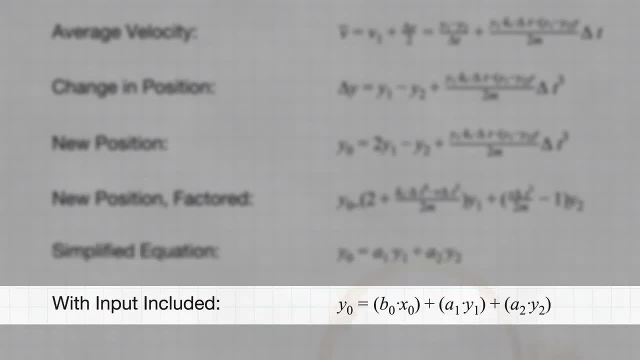 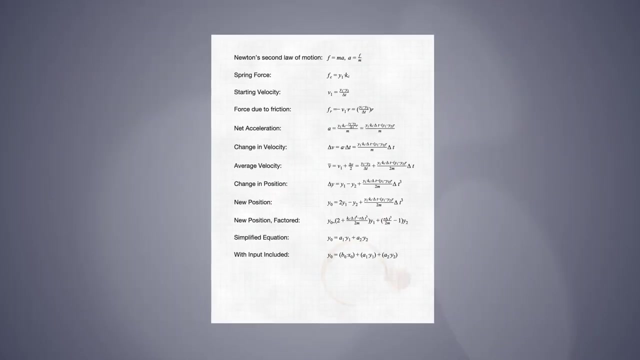 this mathematical model. So all we need to add is one more coefficient, which we'll call b0.. We multiply the current input sample, x0, by b0, and add that to the result. Now we have a complete mathematical model, which. 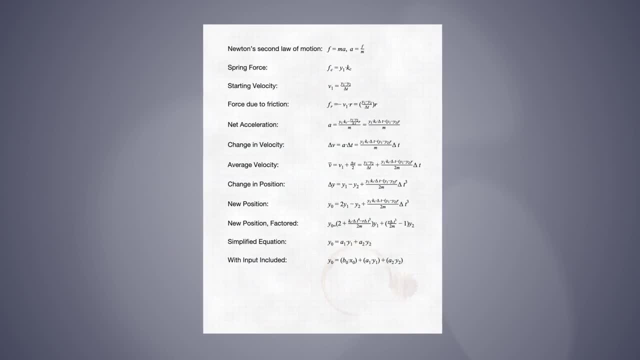 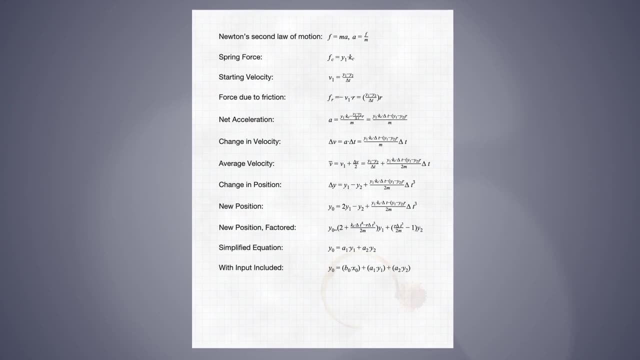 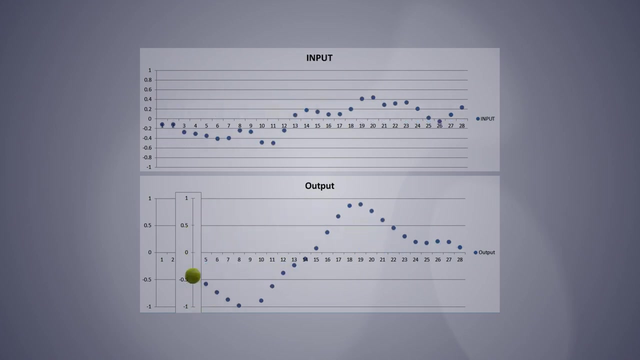 we can use to calculate the result. We can use to calculate the complete response of the ball to any input. It's not just a model that gives us the impulse response, It runs in real time, so it can run on any arbitrary waveform, even, for instance, an audio waveform. 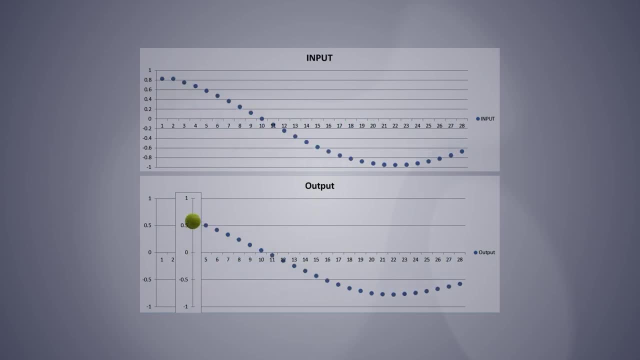 Let's see what happens if we put a sine wave into our system. A very low frequency sine wave passes through essentially unchanged. If we set the frequency to the resonant frequency of our system, the sine wave is actually amplified and at high frequencies there's almost no response. If we step through all of the frequencies. 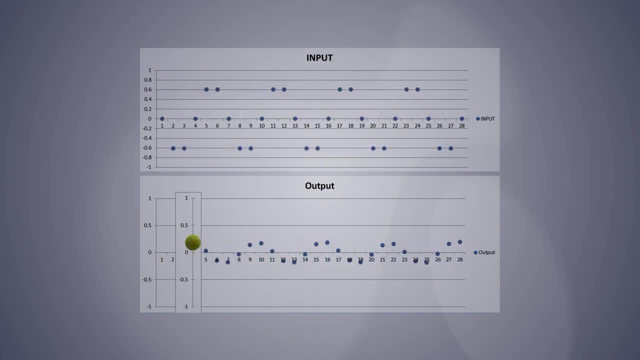 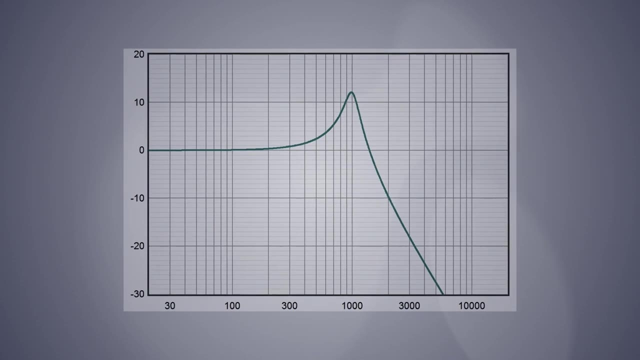 we're interested in, and plot the output level against frequency, we get the frequency response of the system, which looks like this: Well, what do you know? It's an under-damped low-pass filter. Okay, so what does a ball on a spring have to do with audio processing? Well, it's a. 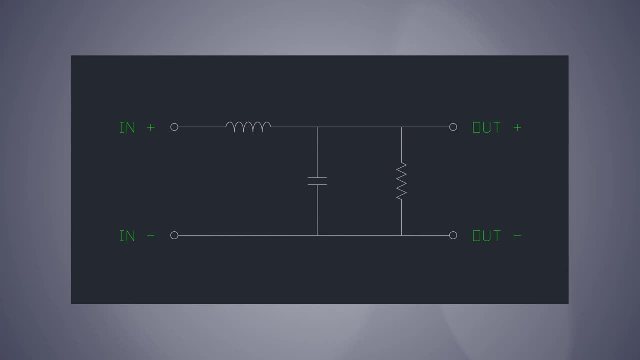 very simple process. We could make an electrical circuit that has the same impulse response as our ball on a spring. The circuit would have an inductor which acts just like the mass of the ball, a capacitor which acts just like the spring, and a resistor which 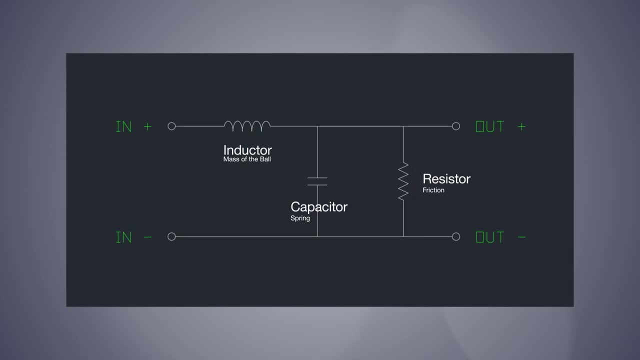 has the same effect as friction. The mathematical model we just built of the ball and spring will also emulate the behavior of the electrical circuit. It would just be modeling voltage and current instead of force and velocity. If we run our little program in real time on an audio stream, we have a digital low-pass. 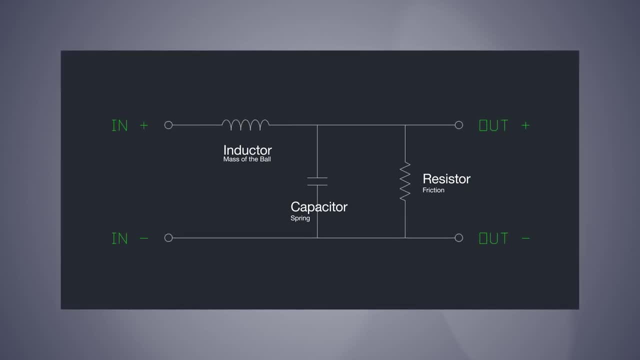 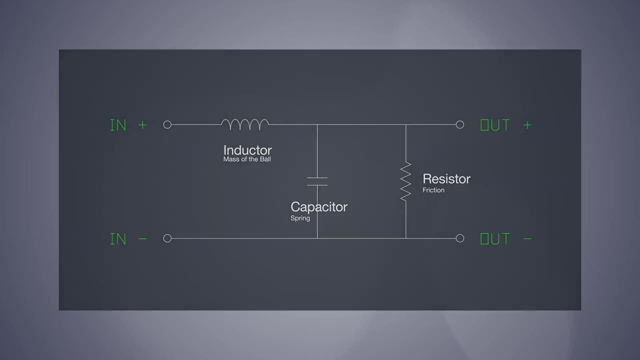 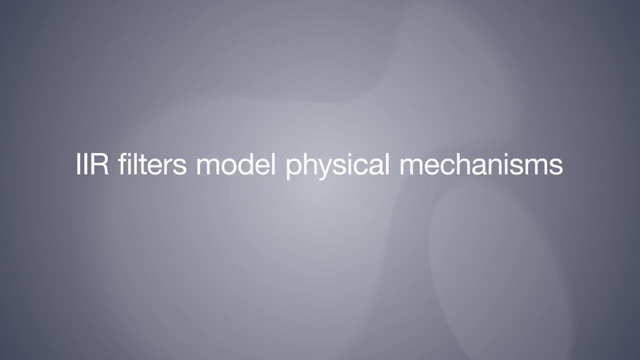 filter. This particular type of filter is called an IIR or infinite impulse response filter, and it's called that because the resonance can theoretically take forever to decay. As we've just seen, an IIR filter actually models the internal mechanisms of a physical. 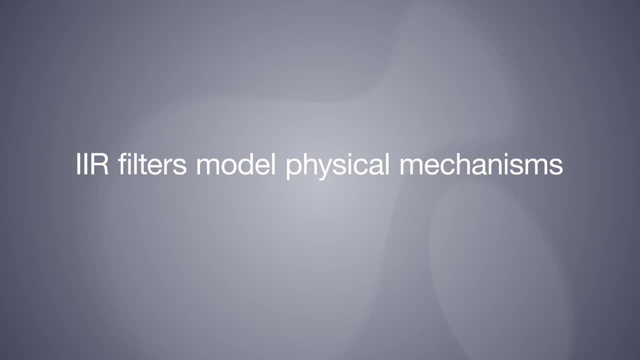 system. It's very handy because you can easily create an IIR filter that can be used to model the internal mechanisms of a physical system. It's very handy because you can easily create an IIR filter that can be used to model the internal mechanisms of a physical system. 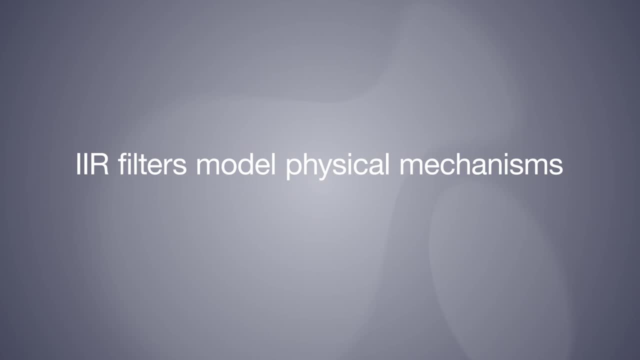 So each filter works the other way too. We can also use our książial IIR filter to emulate any electronic filter you build. The other main type of digital filter is called an FIR, or finite impulse response filter. It works differently than an IIR filter does because it doesn't model the internal mechanisms. 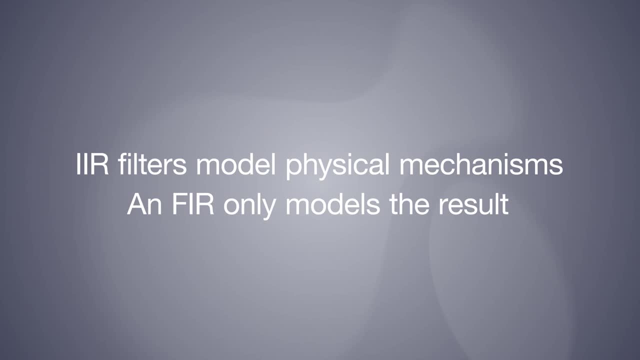 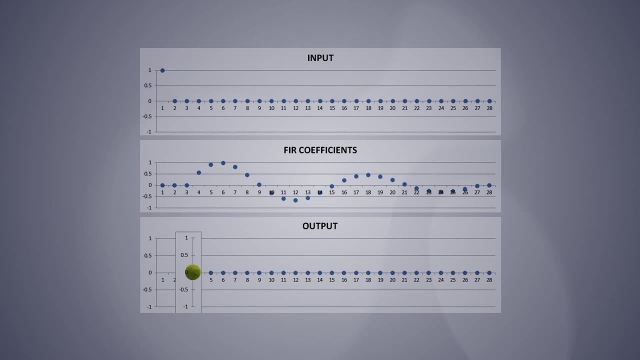 but only models the result. Fundamentally, it does this by only looking at the input stream and ignoring the output stream. All we have to do is take the impulse response of our filter, flip it around backwards and those become our FIR coefficients. 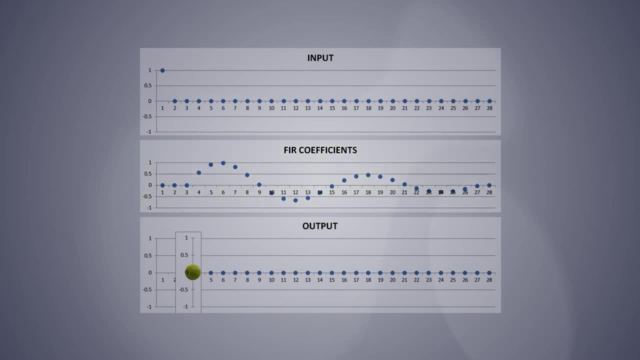 Now, when we want to calculate the next sample, we multiply each of the FIR coefficients by its corresponding input sample, multiply the first coefficient by the current sample, second coefficient by the previous input, and so on and so on. In this example, of course, there's only one non-zero input sample. 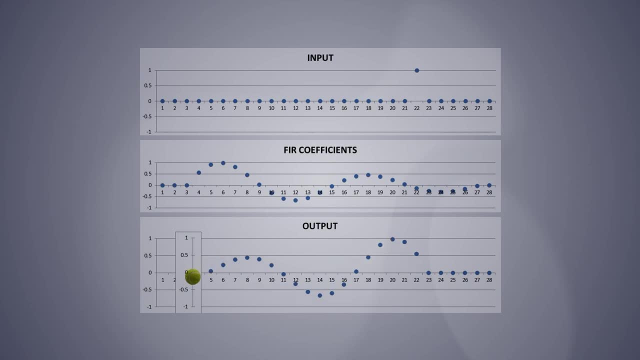 So if I start the filter running, you can see that it simply reproduces the impulse response shape defined by the FIR coefficients. Now, if we keep this running for a while, eventually something different will happen. Well look, the tennis ball stopped. 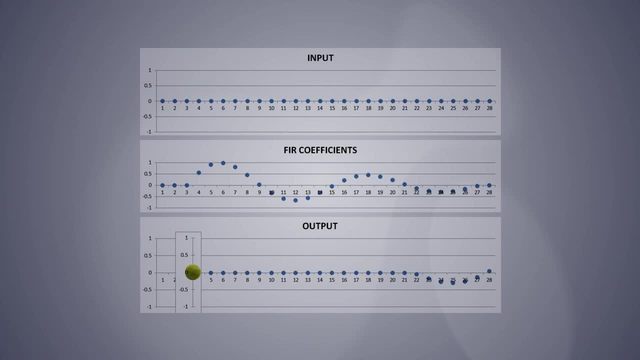 What's up with that? Well, what happened there is that we ran out of FIR coefficients. The impulse response was essentially truncated at that point and that's the finite part of the finite unit. That's the impulse response designation for these filters. 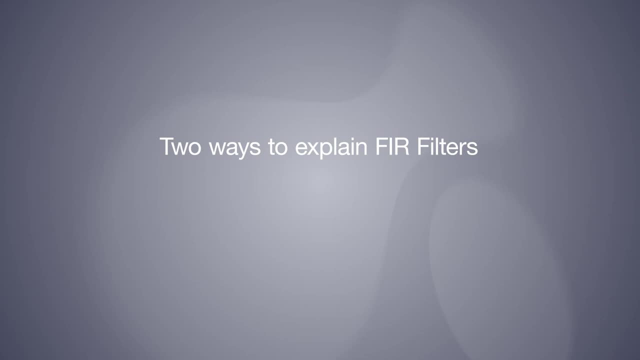 There are two ways to explain what an FIR filter does to a complex signal. One is that each output sample is a weighted average of the recent input samples. That's an easy way to wrap your head around it, but it doesn't really explain much about. 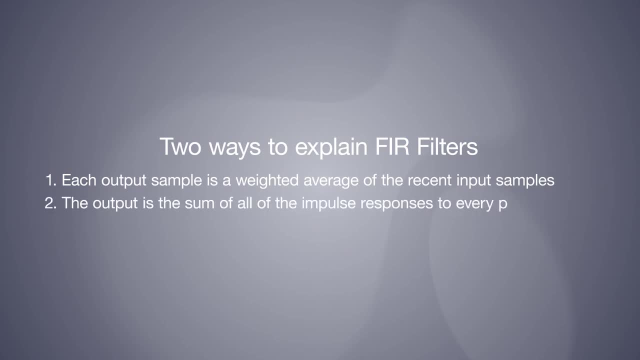 how it works. The second way to look at it is to treat each input sample as an independent impulse. The net output is the sum of all of the impulse responses. For me at least, that connects the impulse response with the filter's response to a complex 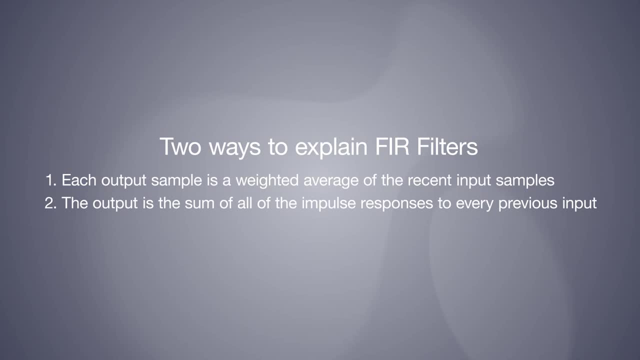 signal. The shape of the signal waveform determines how all of the individual impulses add up. Now that we all know how an FIR filter works- I'm joking, of course- If you didn't already have an understanding of FIR filters, I don't expect you to suddenly. 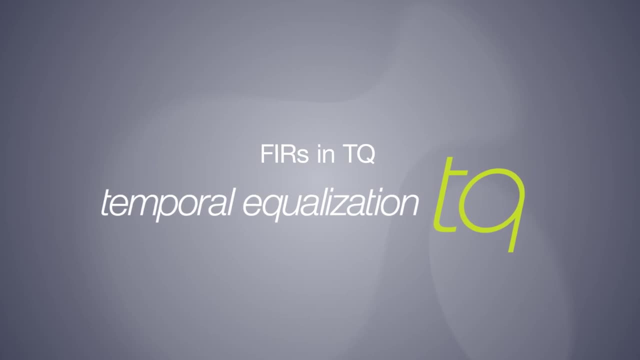 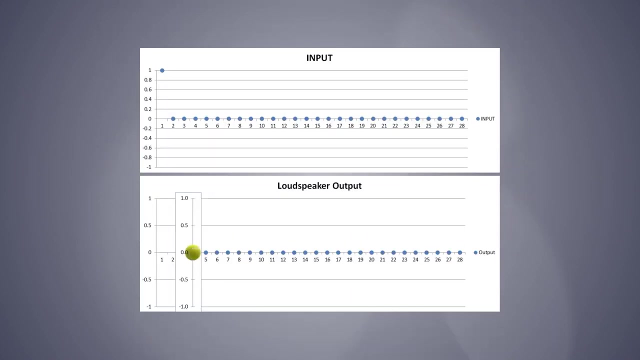 get it from that explanation, but I hope at least that you get what an FIR program does. That's enough for now. Let's look at an example. We'll create an input that is an exponentially decaying string of pulses. This is oversimplified, of course, but it's representative of what a phase plug does to. 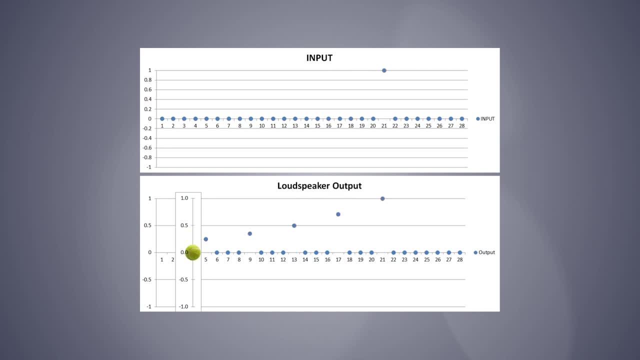 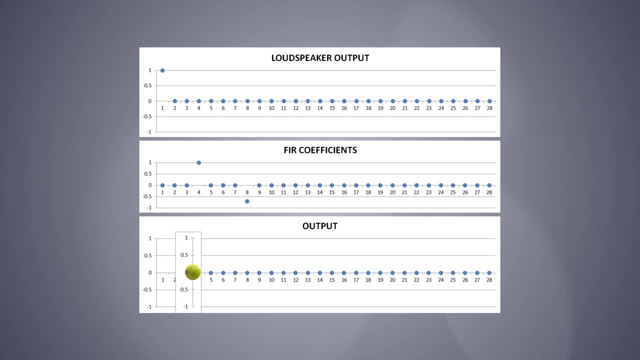 a high-frequency transient, for example, or the resonant decay of a horn or the resonance of a cone. Now what I can do is put in a very simple FIR filter and as we step through the process, you can see that the first impulse passes through. 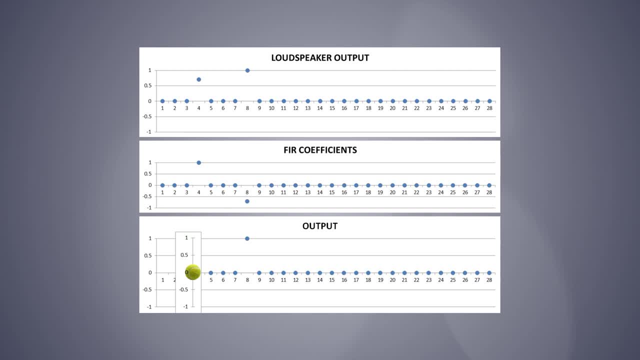 But when the second impulse arrives it's canceled out because the first impulse multiplied by the second FIR coefficient is equal and opposite to the second impulse multiplied by the first FIR coefficient. So they sum to zero. If we continue on from there, you can see that the pattern repeats and the result is: 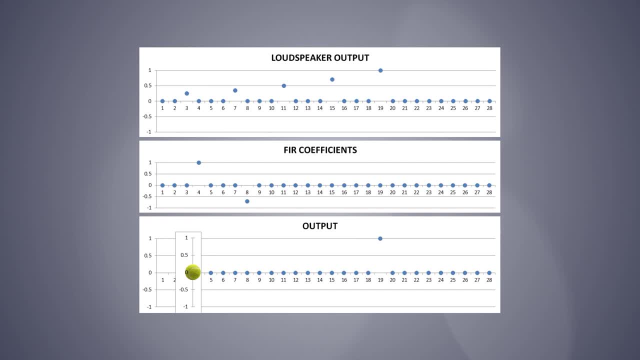 a pure impulse. Of course, there's no way to apply an FIR filter to the acoustical output of a loudspeaker, but the order of these operations doesn't matter. When I was going through math in grade school, they called it the commutative property. 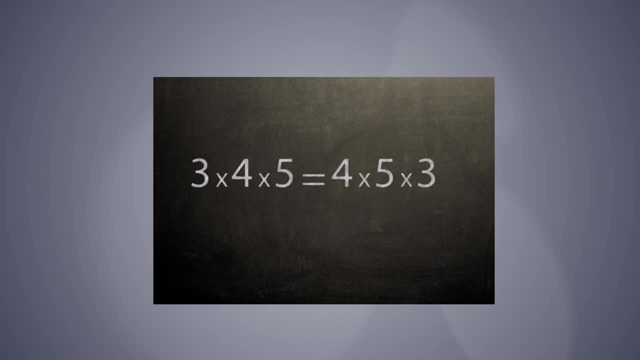 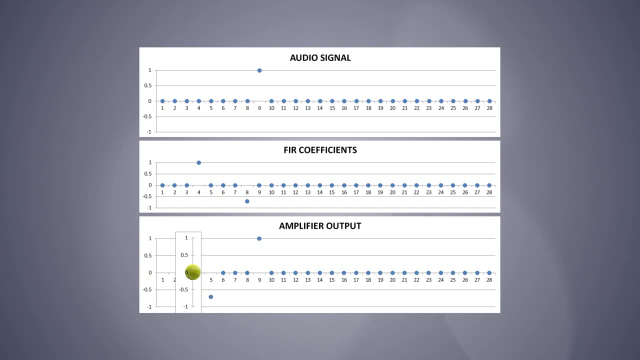 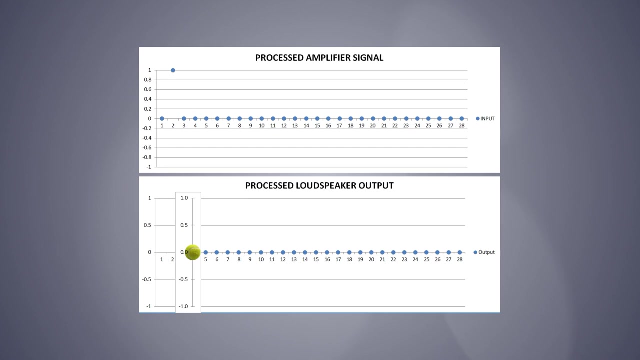 Three times four times five is the same as four times five times three. Filter operations work the same way, So we can move the FIR filter in between the signal source and the amplifier and then notice that the output of the amplifier has time smear now, but the output of the loudspeaker 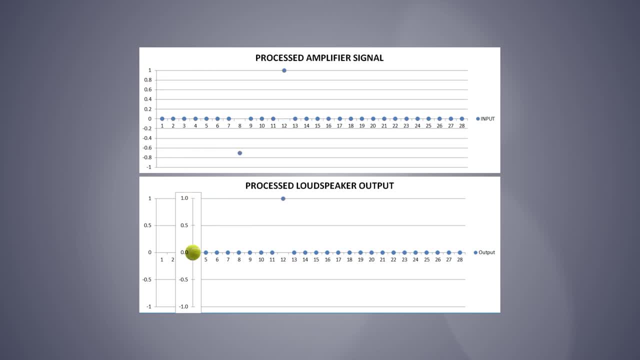 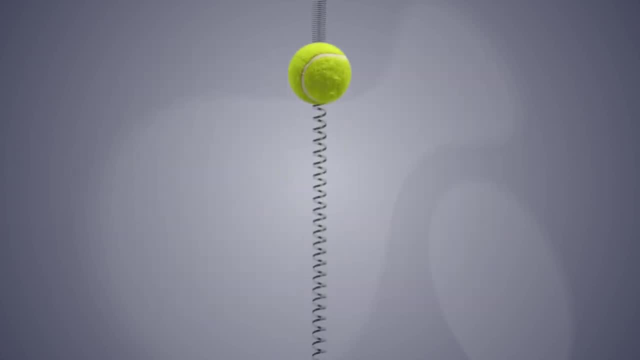 is a pure impulse. That's how an FIR filter can essentially kill a loudspeaker resonance. So there you have it. An IIR filter works by modeling the internal mechanisms of a physical system and is a very efficient way to reproduce what electrical circuits can do. 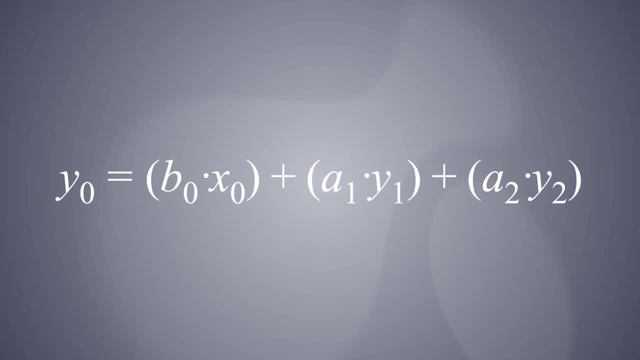 It does it by looking at the input and just a couple of previous output samples. An FIR works by looking at a whole bunch of previous input samples. It's a less efficient way to model a simple circuit, but it can do things that you could.